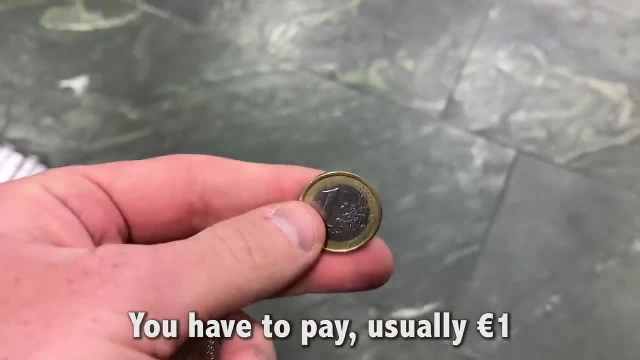 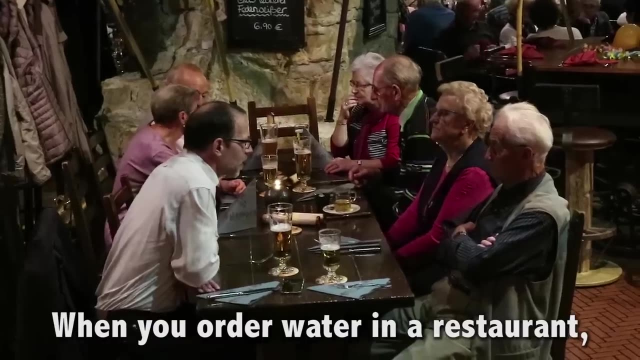 It's not free to pee or do your business in public. You have to pay, usually 1 euro, to use the bathroom, even if it's just to wash your hands. 2. Water is not free. When you order water in a restaurant, it usually comes in a tiny glass bottle and costs 2 to 5 euros. 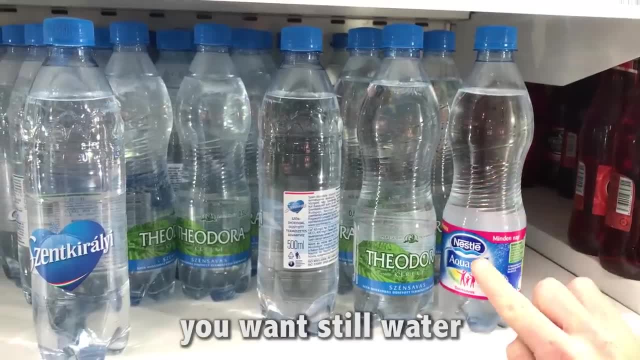 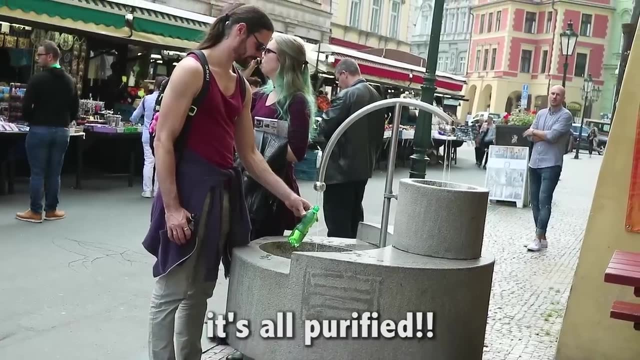 They love sparkling water too, so make sure to tell them you want still water. Can I get a still water, please? Travel tip: Carry around an empty water bottle and fill it up in sinks or public fountains. It's all purified. 3. Every city has history. 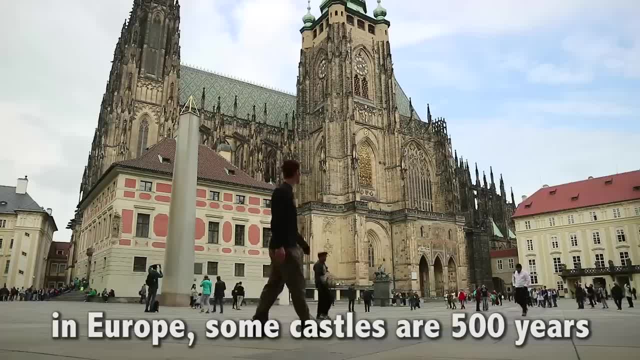 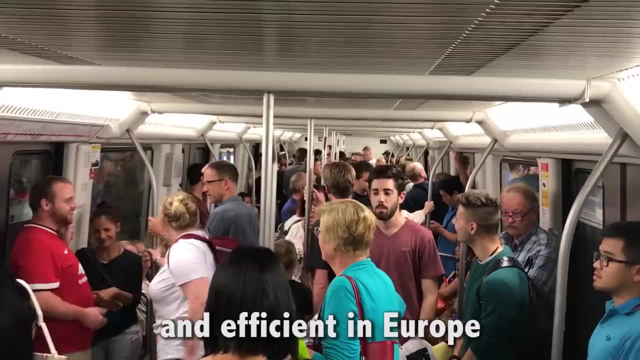 In America we don't have much to talk about before the 17th century. In Europe, some castles are 500 years older than the US even became a country. 4. They drive less. Public transportation is everywhere and efficient in Europe. 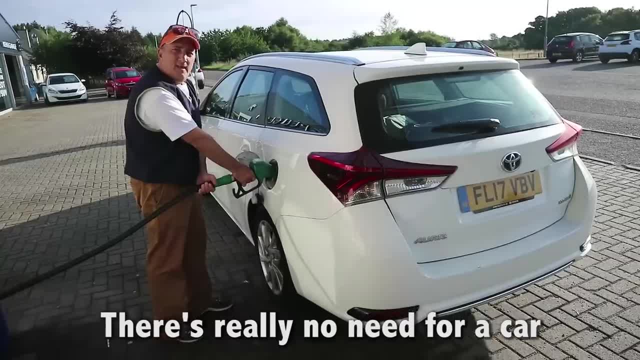 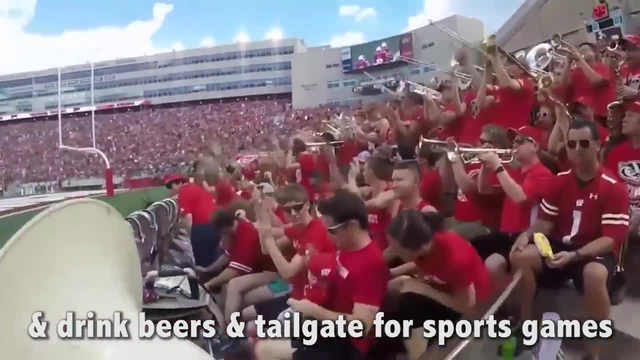 and most cities are pedestrian and bike friendly, There's really no need for a car, and gas is too expensive anyways. 5. Sports are not a family affair. In the States, we pregame and drink beers and tailgate for sports games with our families and friends. 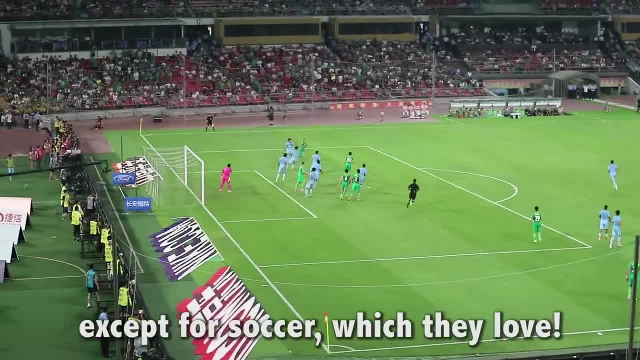 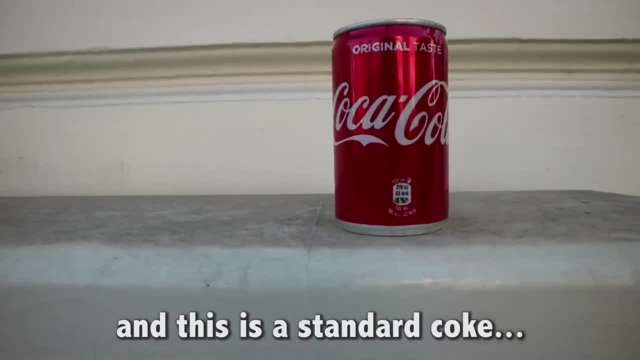 In Europe, sports aren't such big events, except for soccer, which they love. 6. Smaller food portions: This is the size of a normal meal in Europe And this is a standard coke. Also, ketchup is not free and comes in glass bottles. 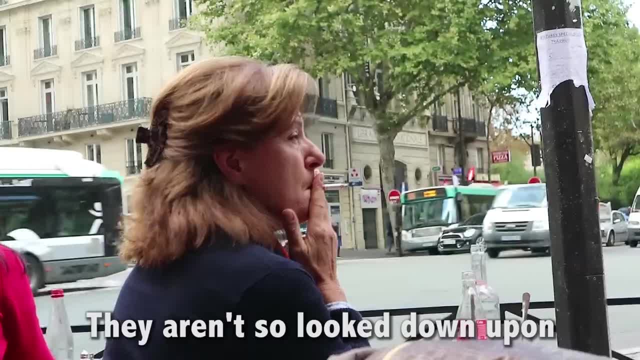 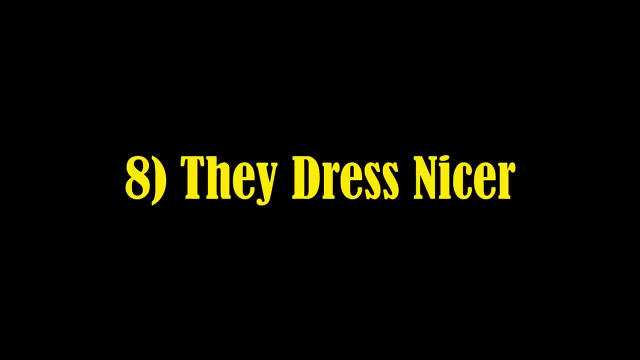 Seriously. 7. Cigarettes are fashionable. They aren't so looked down upon among Europeans either. I guess they don't have the DARE program in Europe. In other words, smoking equals cool. 8. They dress nicer. They don't just throw on basketball shorts, a university t-shirt and sandals. 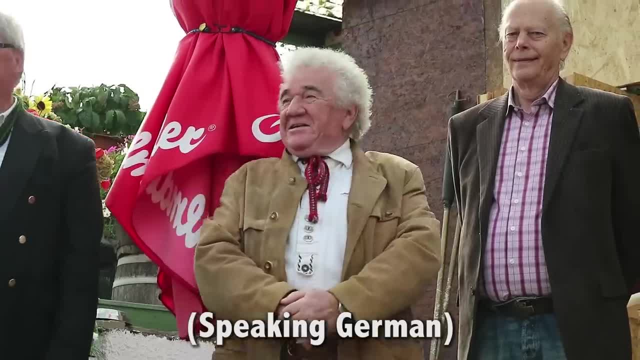 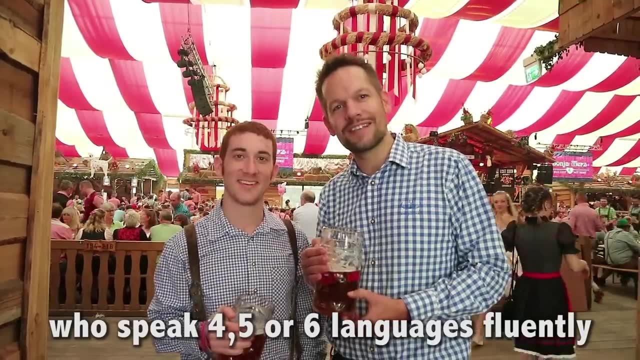 Sup dude. They always dress to impress. And about those haircuts? 9.. They can speak multiple languages. It's not uncommon to meet Europeans who speak 4,, 5, or 6 languages fluently. This beer is very good. 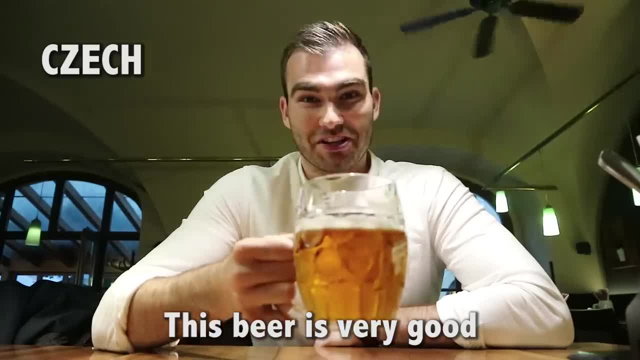 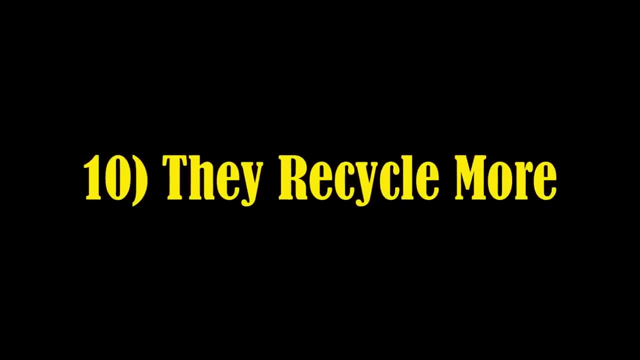 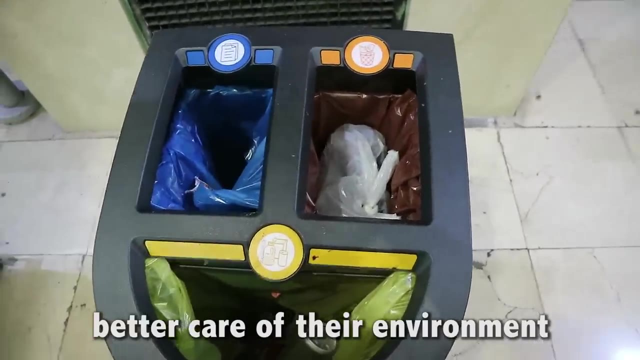 This beer is excellent. This beer is excellent. This beer is very tasty. This beer is very good. 10. They recycle more: Metal cans, plastic, paper bottles. Europeans recycle more and take better care of their environment. In Germany, the government incentivizes you with 25 cents for returning an empty bottle. 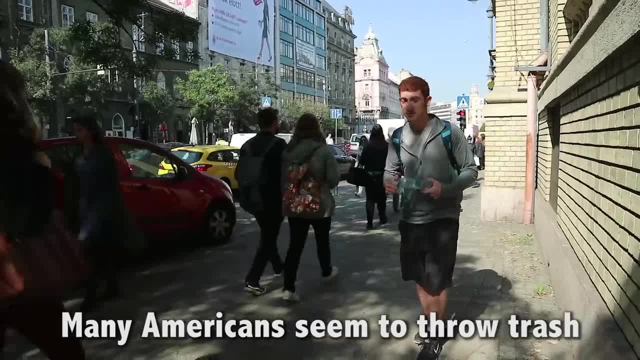 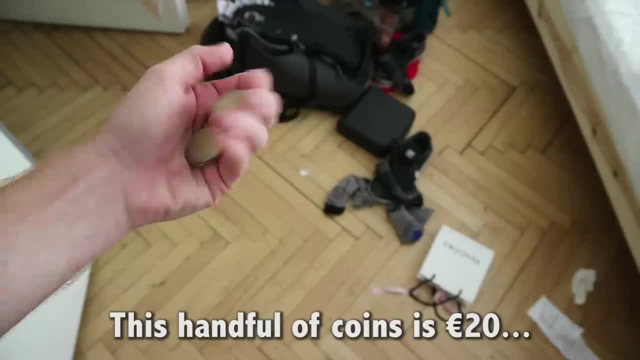 Empty water bottles can make you rich. in Germany, Many Americans seem to throw trash on the streets without thinking about the consequences. 11. Coins actually matter. Don't lose your euros. This handful of coins is 20 euros or 24 US dollars.